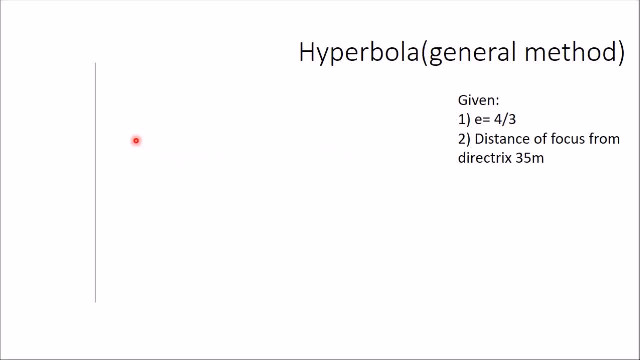 a vertical line as directrix of the hyperbola and in this line mark a point C and from point C draw a horizontal line and in this line mark focus of the hyperbola, which is 35 mm away from the directrix, that is, 35 mm away from point C. So this distance is 35 mm and this point is point F, which is focus of the hyperbola. Now this CF should be divided. 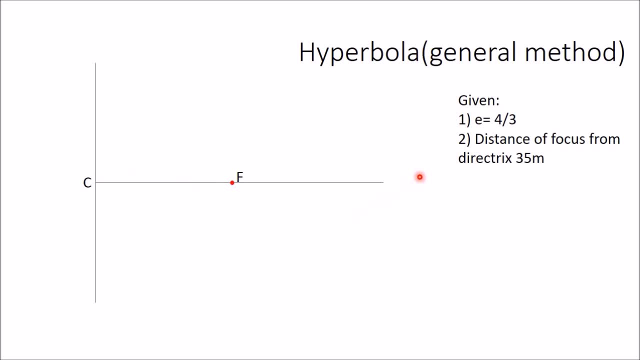 into some equal number of parts. This number of parts depends upon this eccentricity: 4 by 3.. So numerator plus denominator, total number is 4 plus 3, 7.. So divide CF into 7, equal number of parts. After this you have to mark vertex of the hyperbola, which is 4 parts away from F and 3 parts from C. Count from F: 1,, 2,, 3, 4.. So this point should be our vertex of. 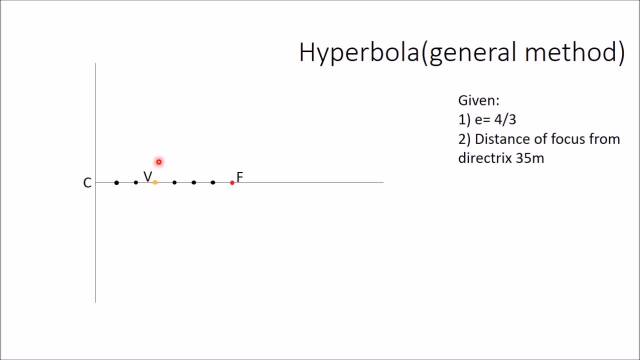 hyperbola. So this point relies on hyperbola, because the ratio of distance of this point from F to C is 4 by 3.. Next step is to draw a vertical line from this vertex V And at the same time draw an arc with center. 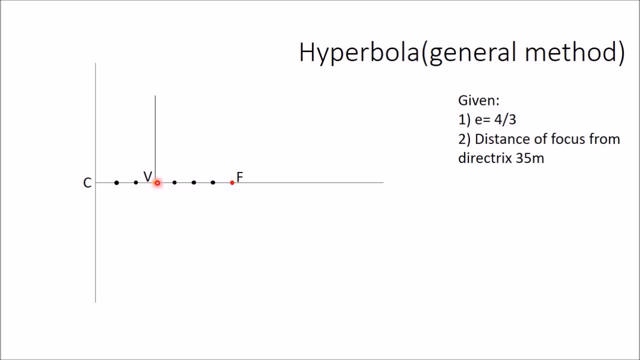 V and distance equal to VF. So center V and distance VF. Draw an arc. This arc is intersecting this vertical line at this point. Mark this point point, join C with this point and extend the line. extend this line now. next, draw vertical lines. 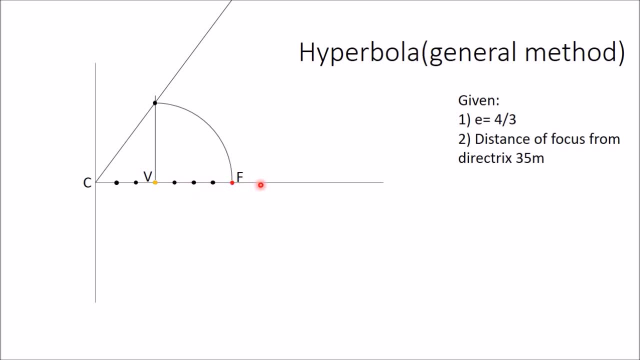 through these points. if space permits, you can take one or two extra points also. you can number these points as 1, 2, 3, etc. and intersection of these vertical lines with this inclined line is 1 dash, 2, dash, etc. now next step is take F as center, 1, 1 dash. as radius. F as center: 1, 1 dash. 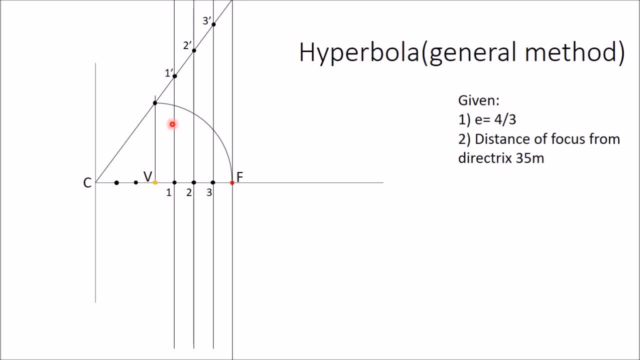 as radius, and draw two arcs which cut this line from one at two places, and these are like this one is this one and another one is this one. so distance is 1, 1 dash and center is F. so in this way you are getting two points of hyperbola same way: 2, 2 dash as distance.